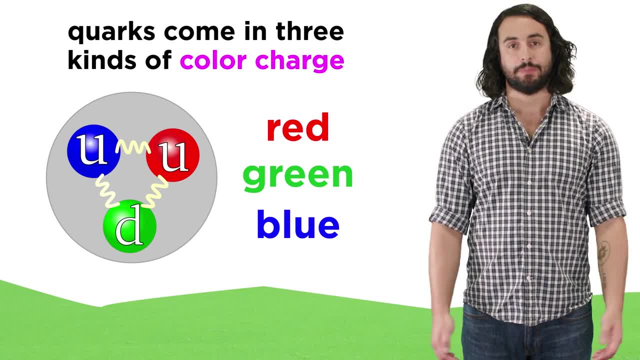 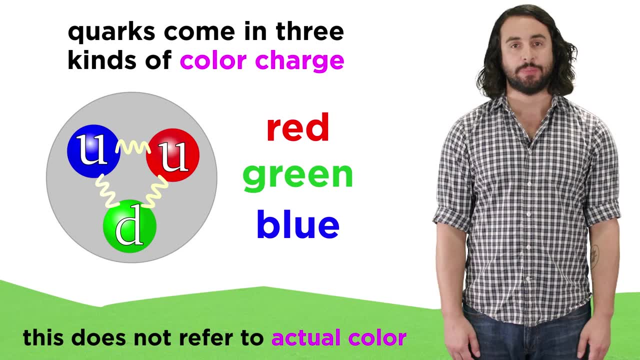 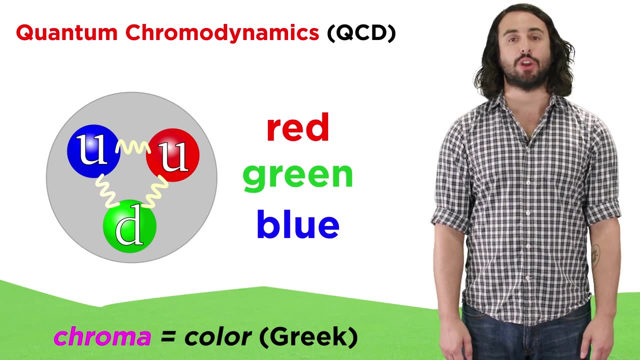 color perceived by humans: Red, green and blue. This does not have anything to do with the actual phenomenon of color. it is just a way of categorizing quarks And since chroma means color in Greek, quantum chromodynamics became the name of the quantum. 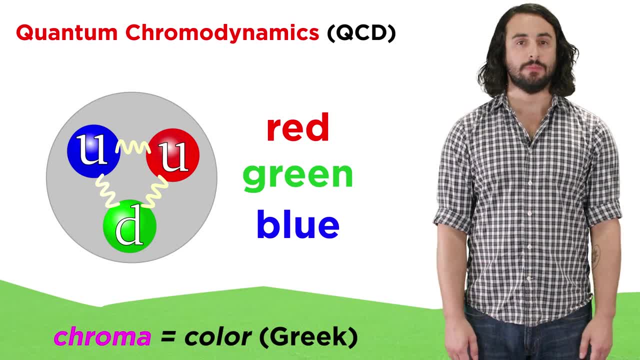 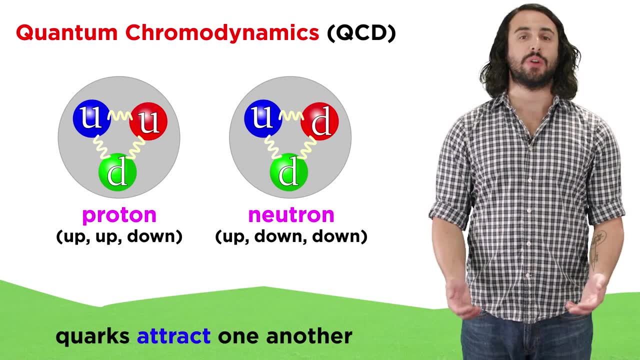 field theory that deals with quarks. Protons and neutrons are each comprised of three quarks which are forever bound. Quarks of different color charge exert an attractive force between one another. They are called quarks of different colors. Quarks of different color charge exert an attractive force between one another. 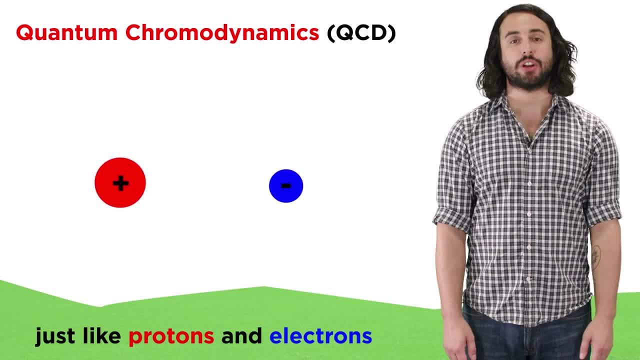 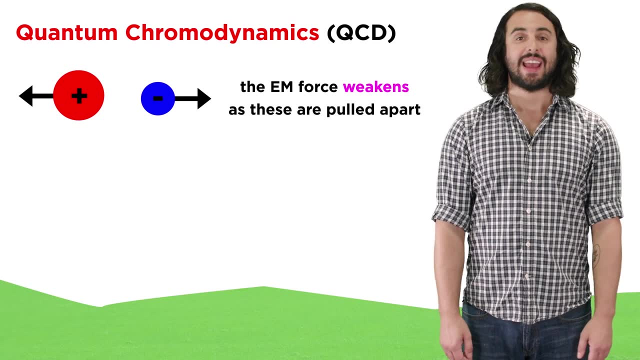 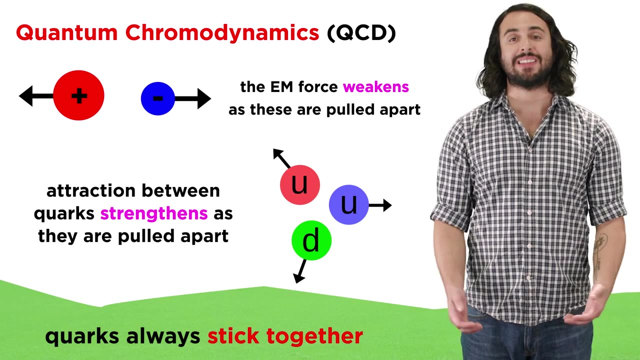 Like the electromagnetic force between particles of opposite electrical charge, But the difference is that the electromagnetic force weakens as particles of like charge are pulled further apart, whereas the attraction between quarks will strengthen as they are pulled apart, so they always stick together. 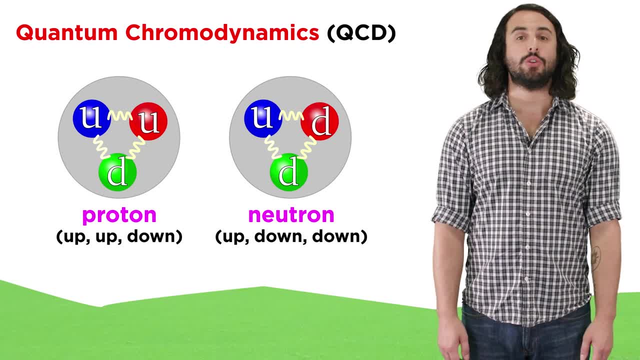 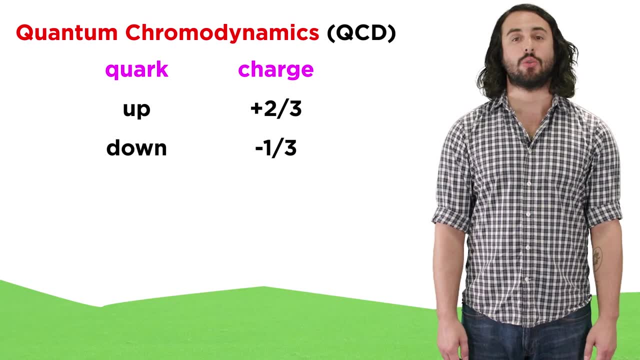 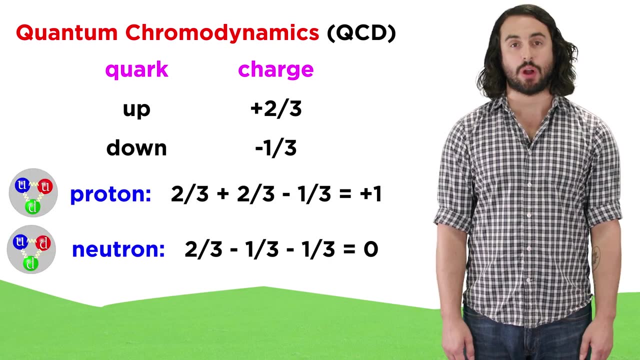 Protons are made of two up quarks and one down quark, while neutrons are made of one up quark and two down quarks. Up quarks have a two-thirds positive charge and down quarks have a one-third negative charge. so, doing the math, we can see how we arrive at plus one and zero as the charges. 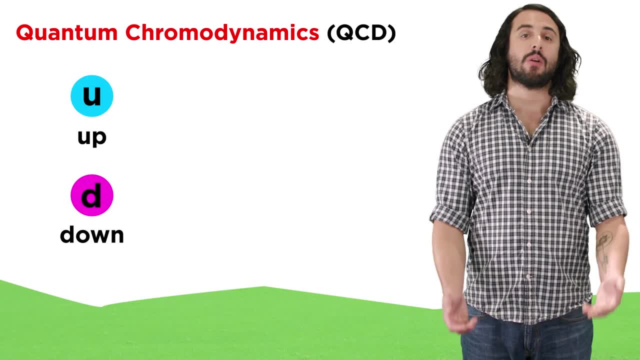 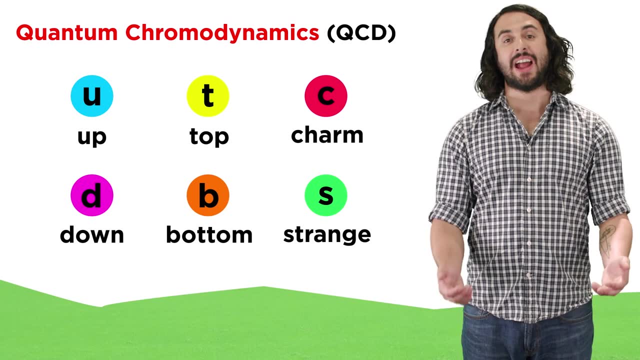 on the proton and neutron. There are other types of quarks. beyond the up and down quark, There are also top, bottom, charm and strange quarks which have different properties. We must understand that the attractive force between quarks is the same as the positive. 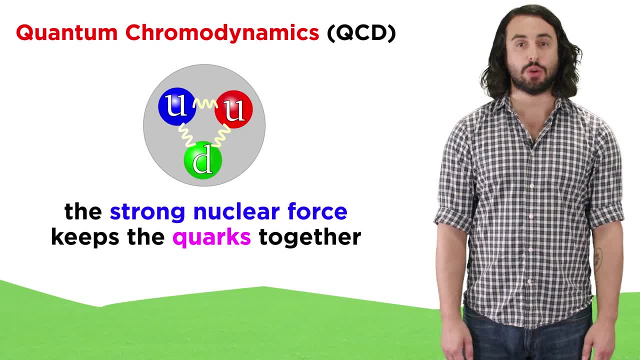 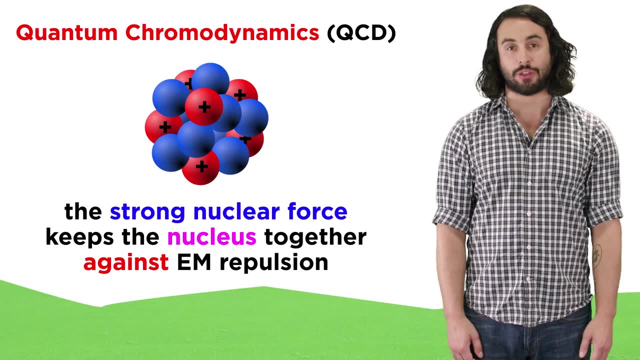 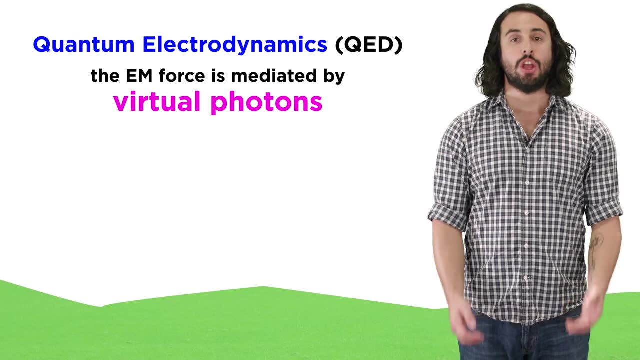 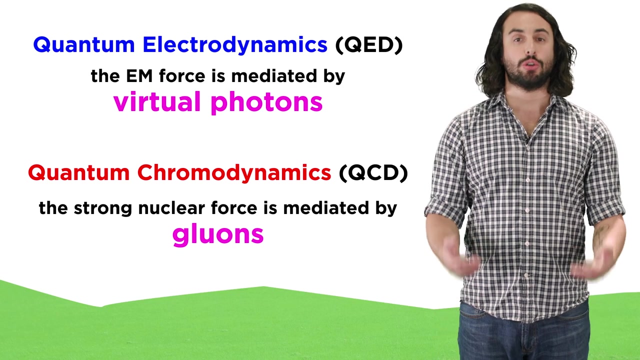 force between quarks. It is the strong nuclear force capable of keeping positively charged protons together against their electromagnetic repulsion. And just like QED did for the electromagnetic force, QCD shows that the strong nuclear force is mediated by the exchange of quanta called gluons. 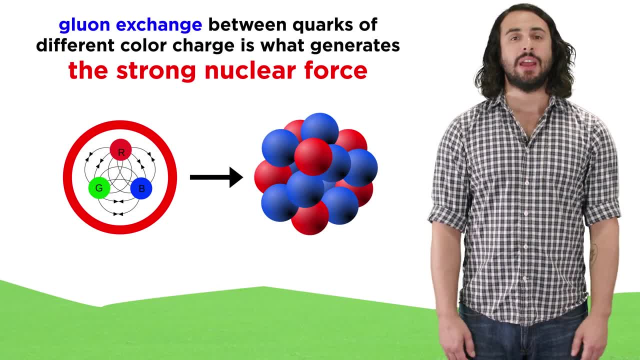 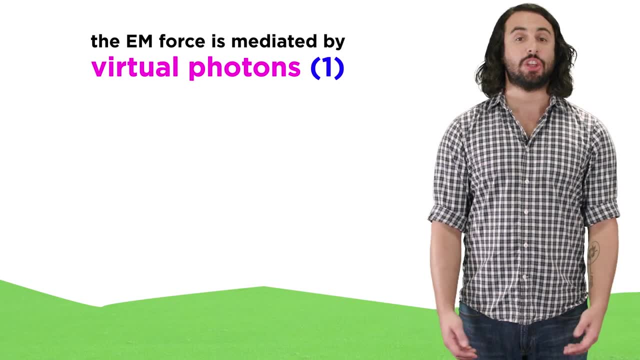 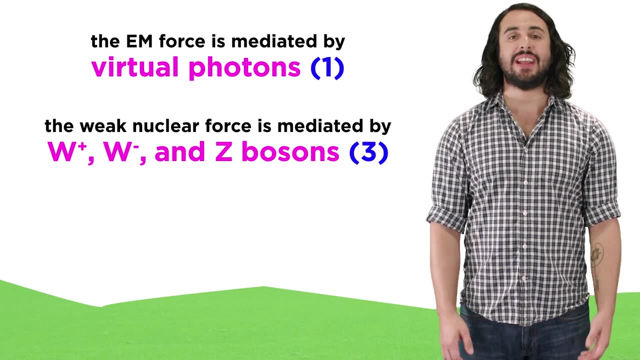 It is the exchange of these gluons, which come in eight varieties, that keeps an atomic nucleus stable. We can see that our quantum field theories are getting more complicated. as QED needed just one particle, the photon, The quantum field theory that governs the weak nuclear force needs three particles.